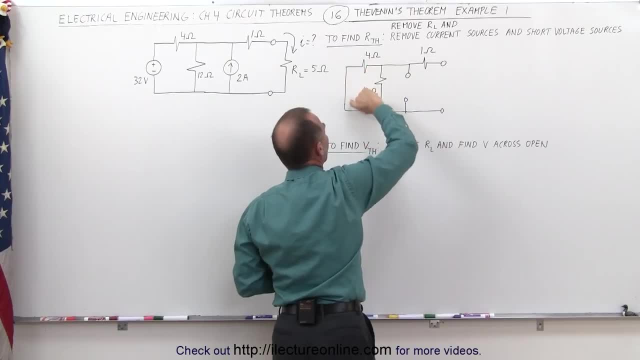 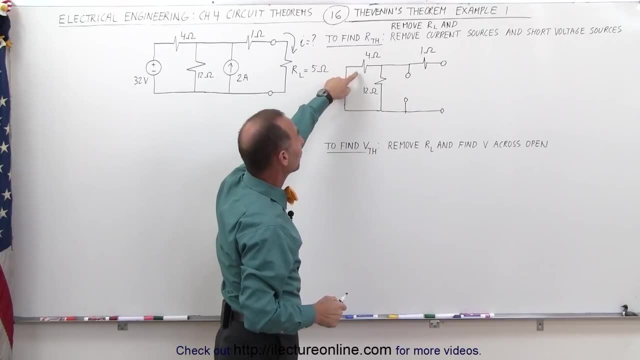 in the circuit. This is in series. These are two in parallel, so let's turn this into a single resistor, Since they're in parallel. the resistance here would be the product of the sum 4 times 12 is 48.. 4 plus 12 is 16.. 48 divided by 16 is 3.. So these two resistors can be replaced by a. 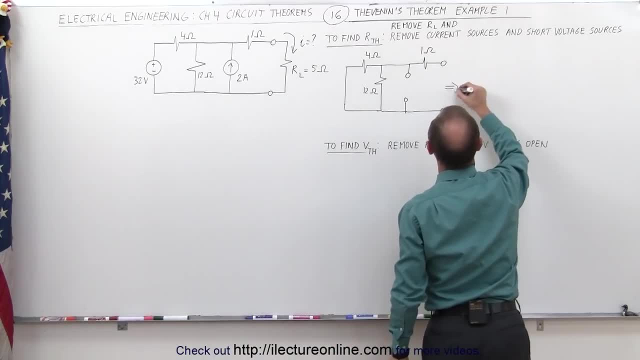 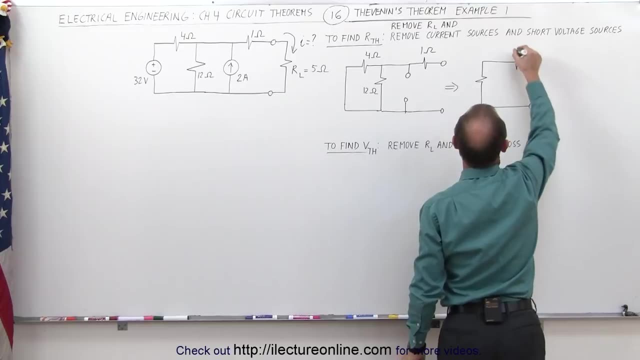 single three ohm resistor. The circuit then becomes the following: We have the one ohm resistor, We have then the three ohm resistor and back to here. So one ohm, the four and the 12 combined become a three ohm resistor, which then turns into: 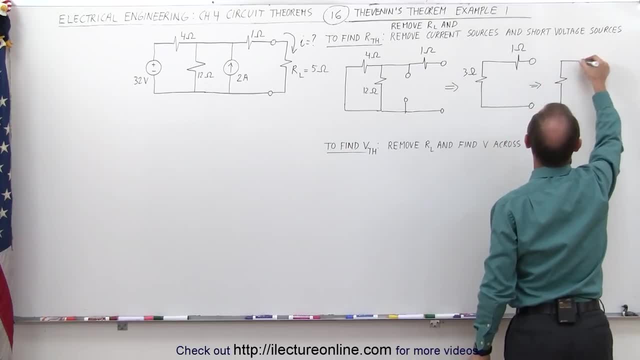 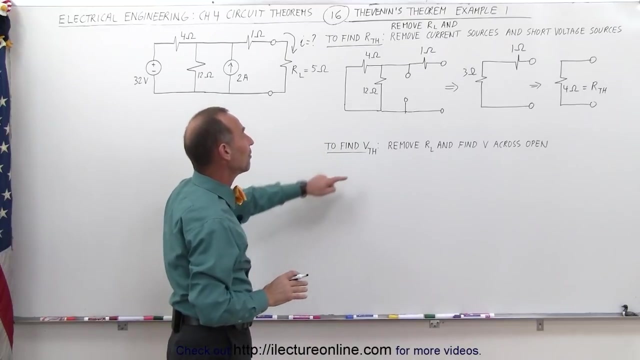 a single resistor, Since those two are in series. add them together and you get a four ohm resistor. That is the Thevenin's resistance. This is R Thevenin. All right, now we've gotten half of the problem. We've got the resistance. Now we need to find the voltage across the open. What? 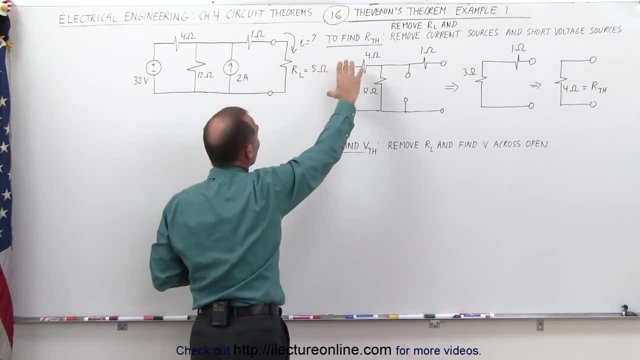 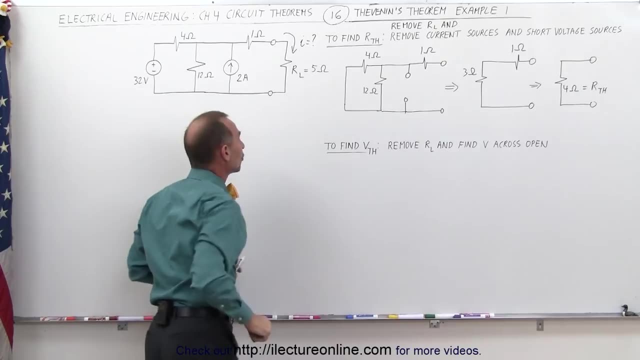 we're going to do to find the Thevenin voltage. again, we remove the low resistor and then we try to find the voltage across what's remaining, by keeping the voltage across the open. We're going to use a one ohm resistor, a two ohm resistor, which they are, Mind you, I want now the voltage. 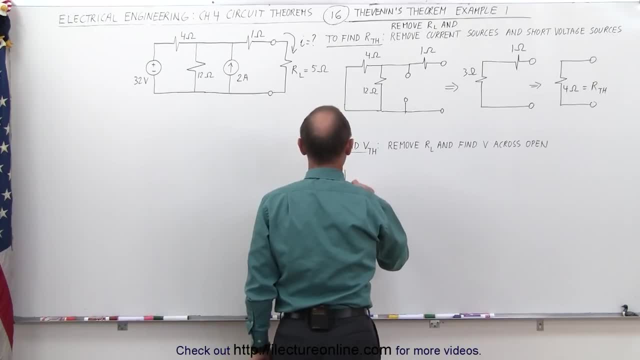 source and the current source in the circuit. So let's go ahead and do that and see what we get. So the circuit becomes as follows: We still have the voltage source in there, We have the four-ohm resistor, Now the 12 Ohm resistor. This is plus minus 32 volts. Four ohms, 12 ohms. 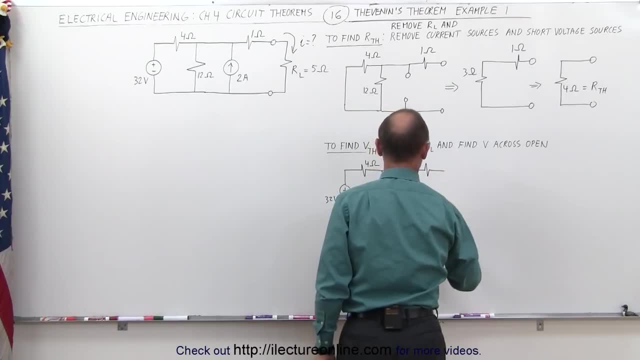 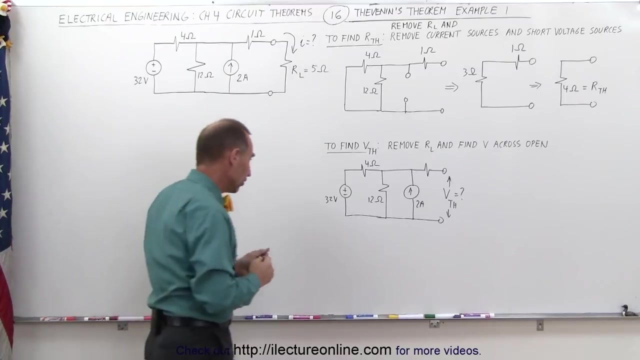 and we have the 1-ohm resistor here, And what is the voltage devonant across here? That's what we're trying to find. How do we do that? Well, we can go ahead and use a node analysis method. 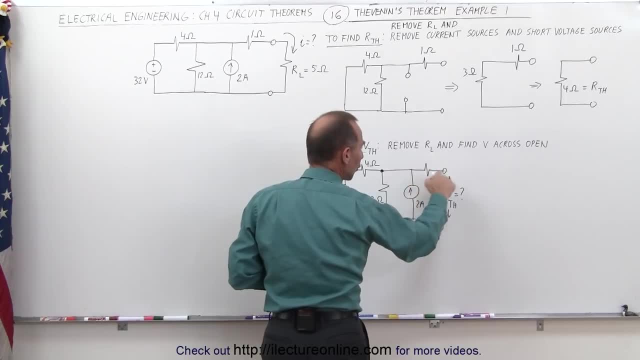 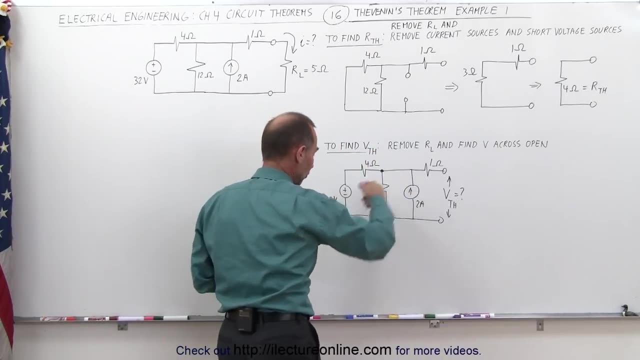 Let's take this node right here. Notice that there's no current flowing through this appendage right here, so the 1-ohm resistor just sits there and carries no current. The current is only in these two meshes right here, So we have a current coming in this direction. 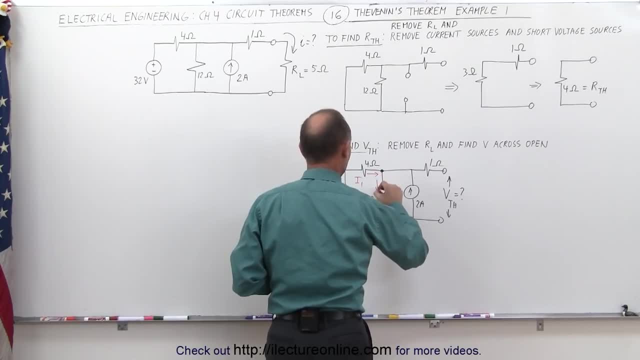 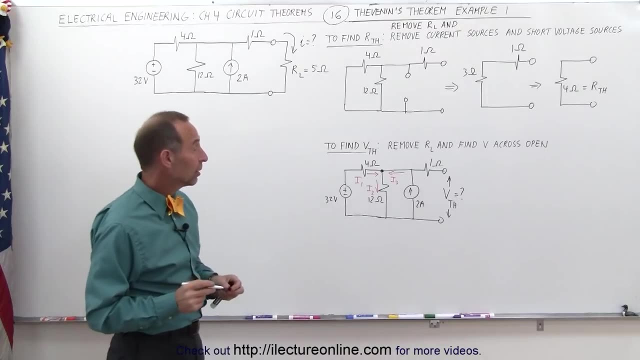 Let's call this I1.. We have a current leaving that. Let's call it I2, and we have a current entering here. Let's call that I3. And using Kirchhoff's rules on currents at a node, we can say that all the currents entering the node 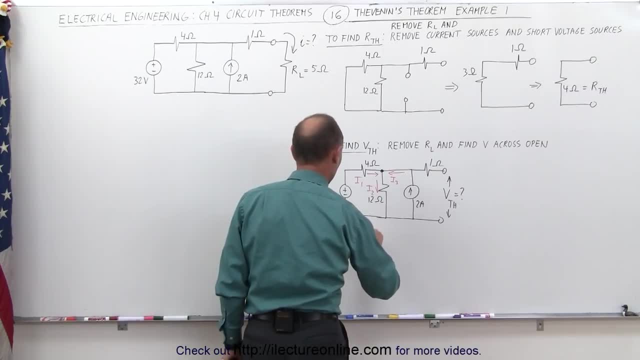 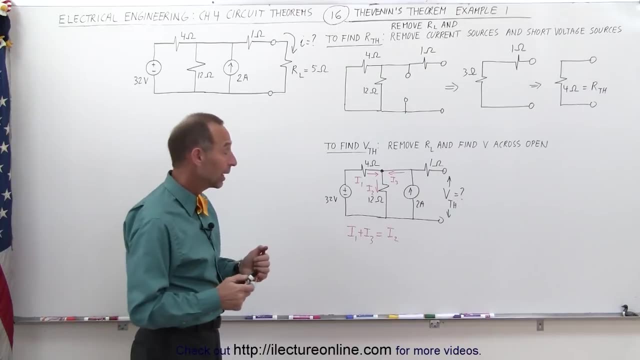 must equal all the currents leaving the node, which means I1 plus I3, those are both entering must equal I2, which is I2.. Leaving the node, Now I'm going ahead and replacing what those are equal to. I1 will be the difference between this voltage, right here, 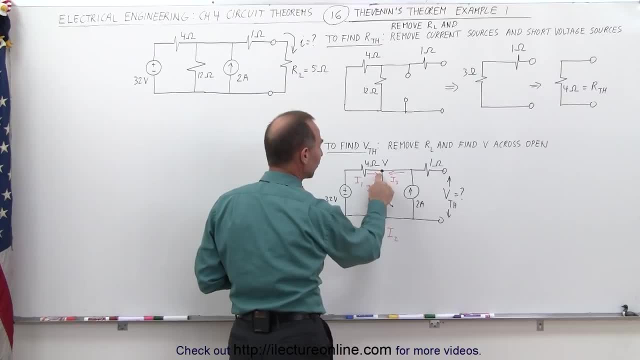 So let's say that this is the voltage we're looking for. Notice that this voltage will be the same as the voltage over there, and this voltage here will be the same as the voltage over there. So this will, in essence, become the Thevenin voltage. 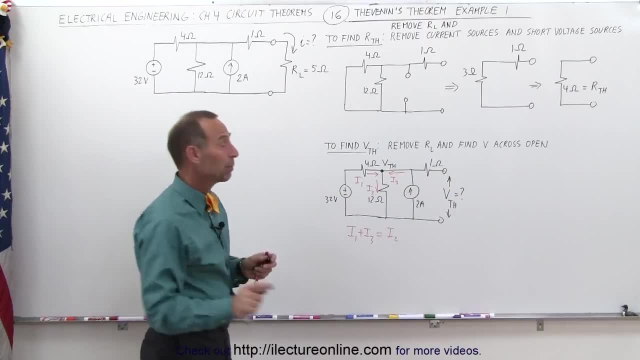 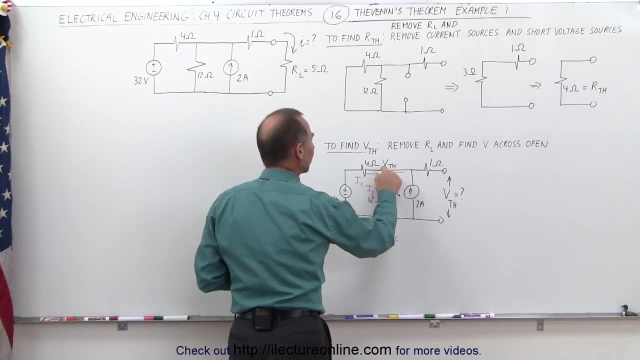 because it's the same as the voltage across the gap there. Remember, there's no current flowing through the 1-ohm resistor, so it's like it's not even there. 32 volts minus V Thevenin divided by the resistance between the two. 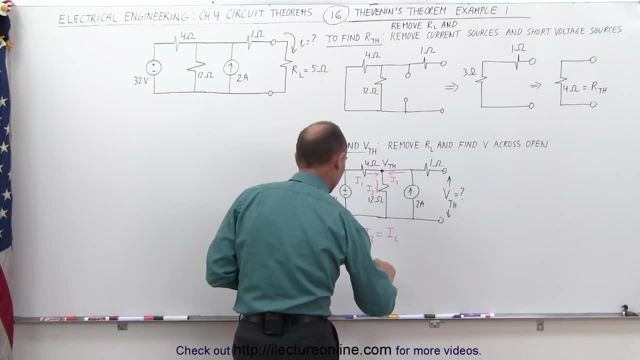 which is 4, that will be the current I1 plus current I3,, which is the 2-amp current entering that node plus 2 equals the current I2,, which is the current from this location to here. That will be the voltage difference, which is V Thevenin. 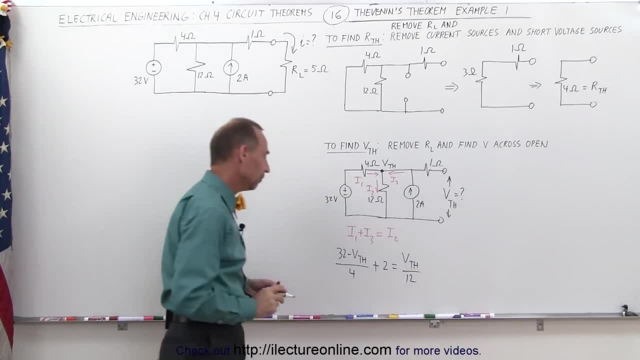 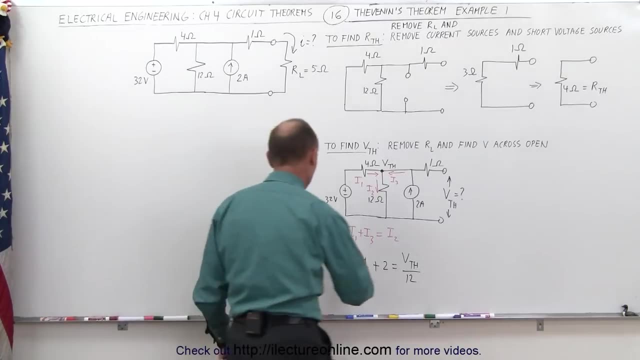 divided by the resistance, which is 12.. All I have to do now is solve that equation for the Thevenin voltage. I can do that by multiplying both sides of the equation by 12.. When I do that, 4 goes into 12 three times. 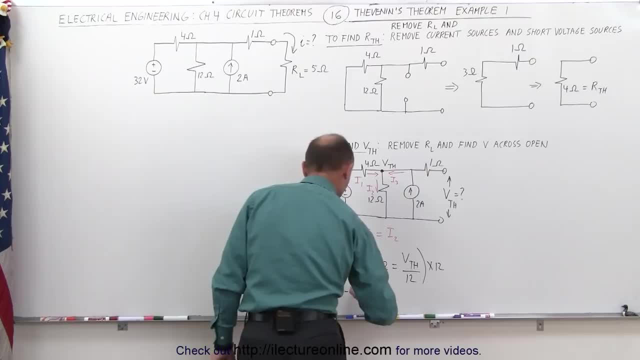 3 times 32 is 96, minus 3 times Thevenin. voltage 3V. Thevenin plus 2 times 12, which is 24, equals the 12th. cancel out, I get voltage Thevenin. 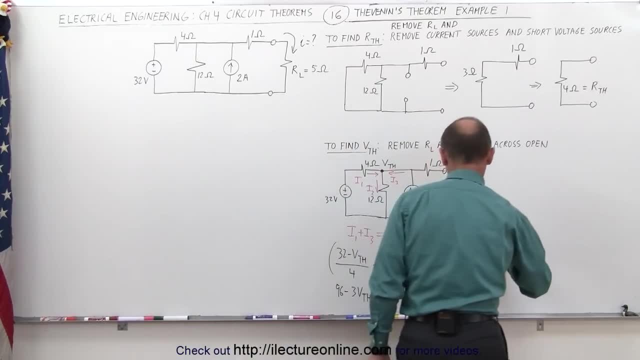 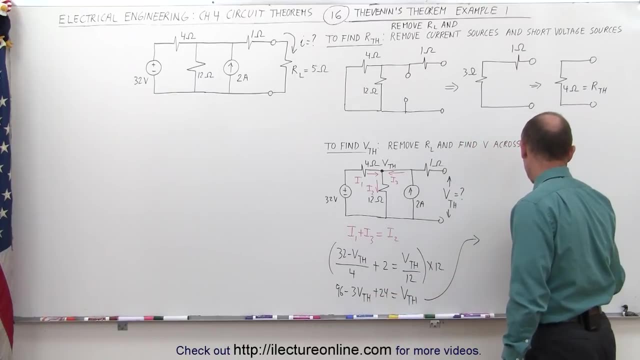 When I move all the voltage Thevenin over to one side- let's come over here And continue. So minus 3 goes, the other side becomes plus 3 plus Thevenin voltage, which is 4 times voltage Thevenin. 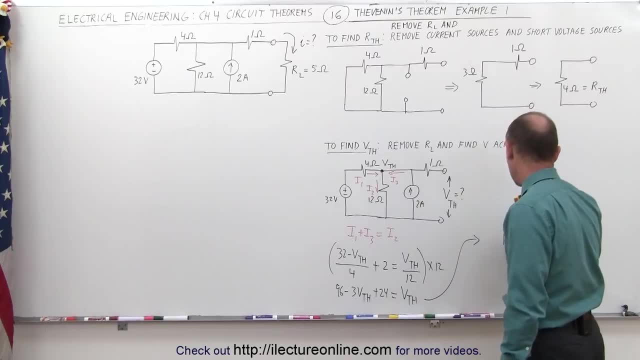 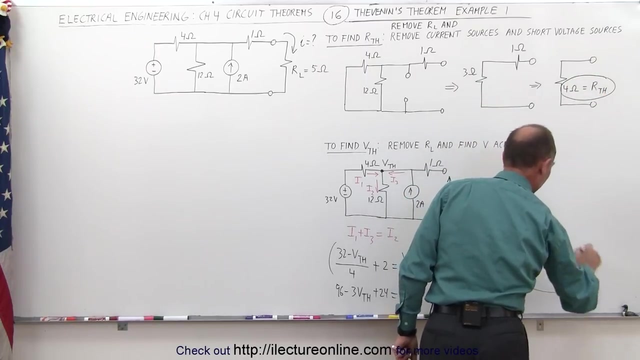 And then on the left side, 96 plus 24,, that's 120.. And that means that V Thevenin is equal to 120 divided by 4, which is equal to 30 volts. So now I have the Thevenin resistance and I have the Thevenin voltage. 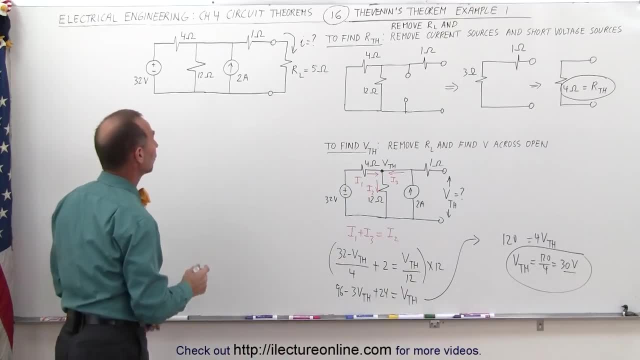 I can now go ahead and draw. I can now go ahead and draw The equivalent circuit. this whole circuit can now be replaced by a single voltage source, which is the Thevenin voltage, V- Thevenin, and a single resistor, which is the R Thevenin. 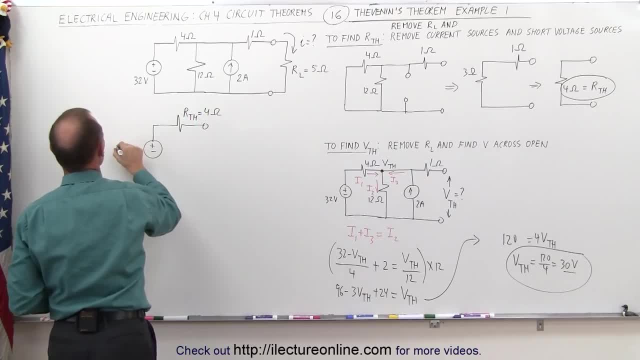 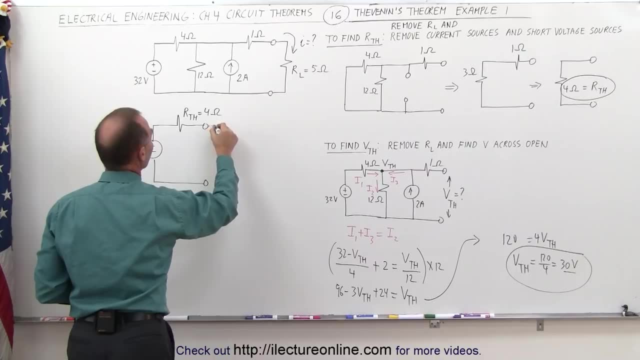 Now R Thevenin is going to be 4 ohms and V Thevenin is going to be equal to 30 volts. And now to that we add the load resistor. Now we go ahead and add it like this: And we said that the load resistor RL is equal to 5 ohms. 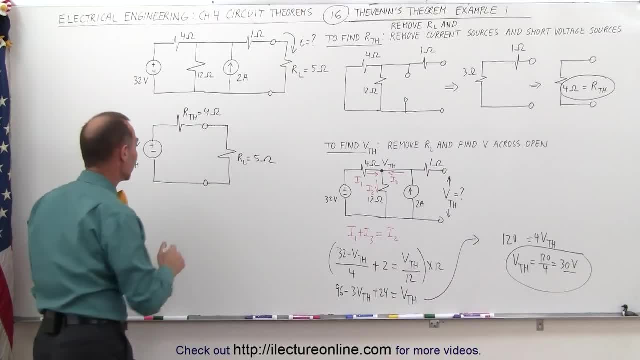 And now we're ready to find the current. because the current is now easy to find, The current I is equal to V divided by the total resistance. That will be the Thevenin voltage of 30 volts divided by the total resistance of 4 plus 5 ohms. 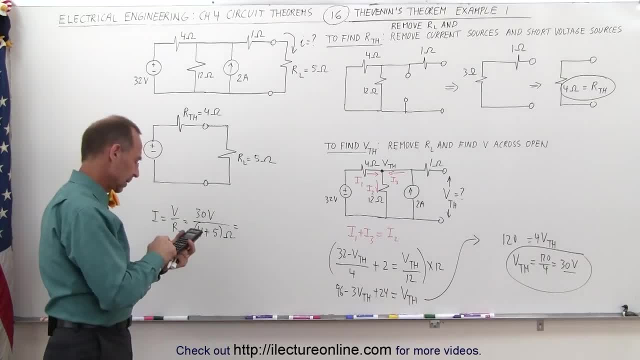 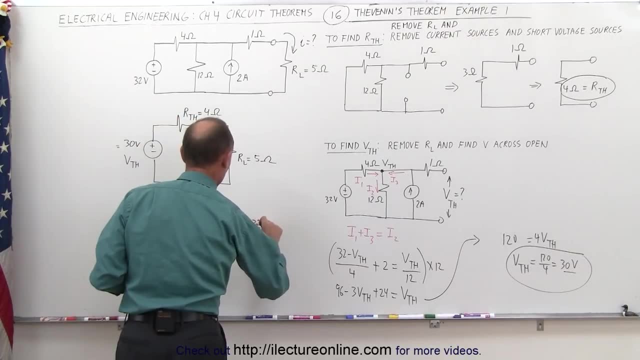 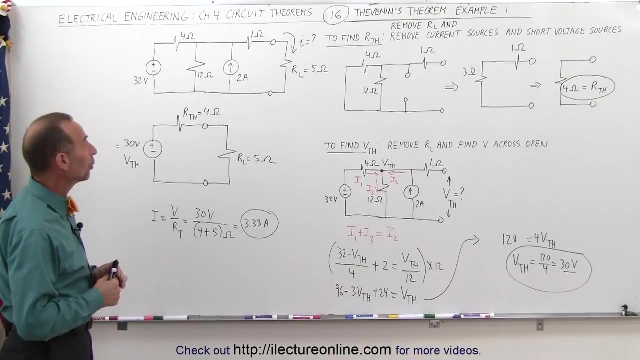 And 30 divided by 9.. 30 divided by 9 equals 3.33 amps. 3.33 amps And that would be the current going through the load resistor. Notice how easy it makes the problem. All we have to do is convert our linear circuit. 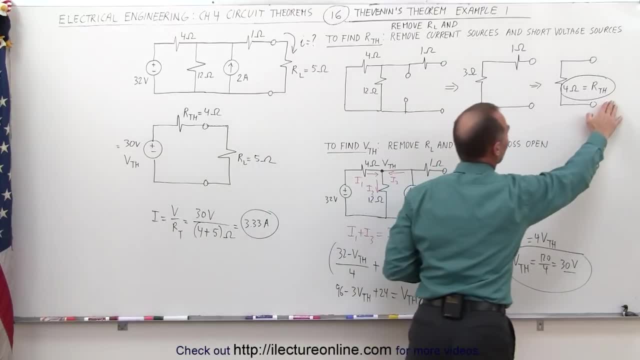 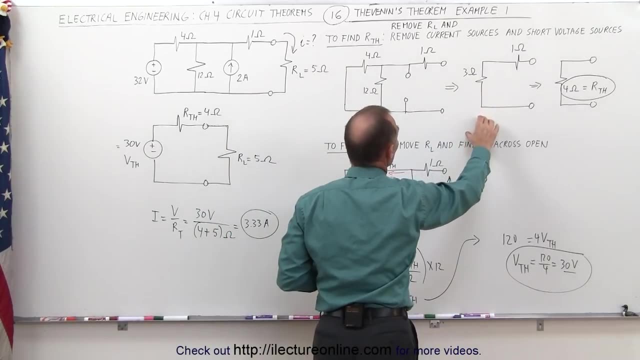 into the Thevenin circuit by finding the Thevenin's resistance and the Thevenin's voltage. Method again to find the Thevenin resistance is: remove the load resistor, We remove any current sources and we short out any voltage sources. 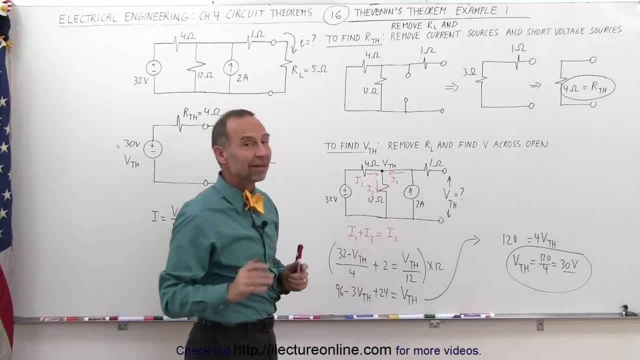 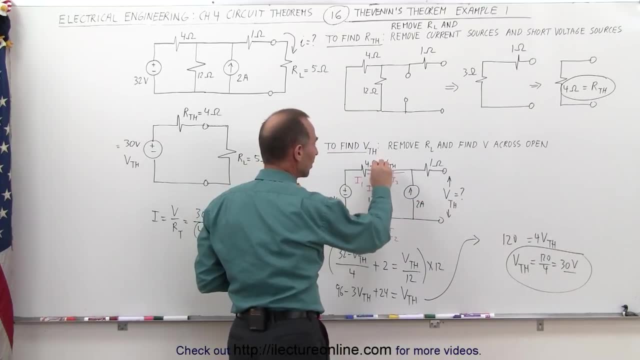 Then we calculate the resistance of the remaining circuit. That becomes the Thevenin resistance, And for the voltages we remove the load resistor And then we solve for the Thevenin voltage using whatever method is convenient. At this point it was convenient to use the node analysis method. 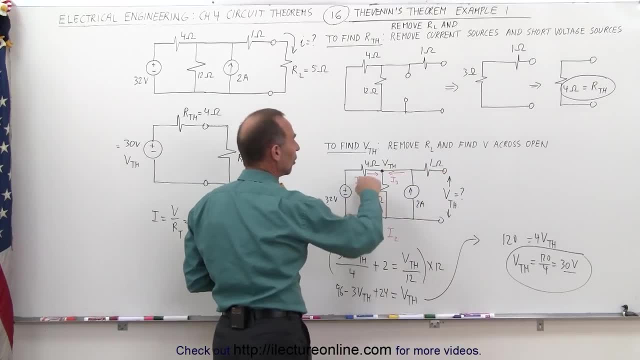 We found this to be the voltage, the same voltage as the Thevenin voltage. We added all the currents that enter and all the currents that leave, set equal to all the currents that leave, And we solve for the Thevenin voltage that way. 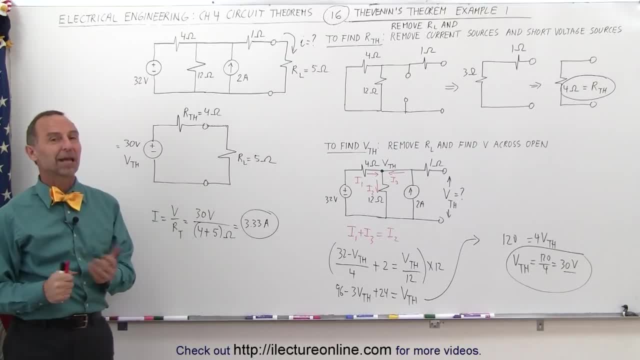 Once you have the equivalent circuit, the rest is really easy, And that's how it's done. That's how it's done.